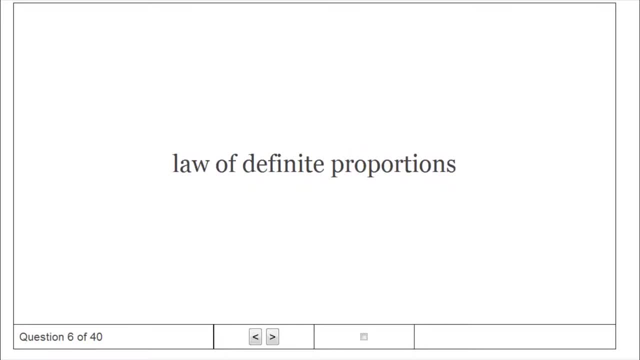 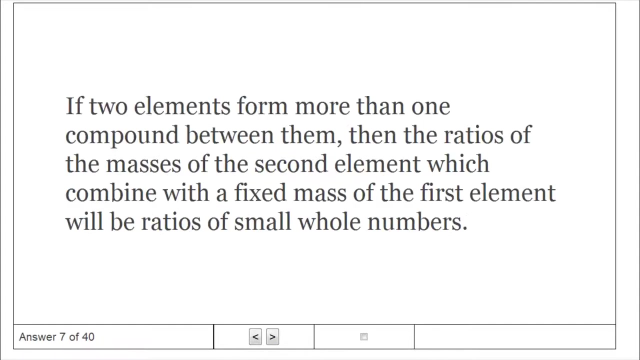 Law of Definite Proportions, Sometimes called Proust's Law, states that a chemical compound always contains exactly the same proportion of elements. by mass Dalton's Law, If two elements form more than one compound between them, then the ratio of the two elements is equal. 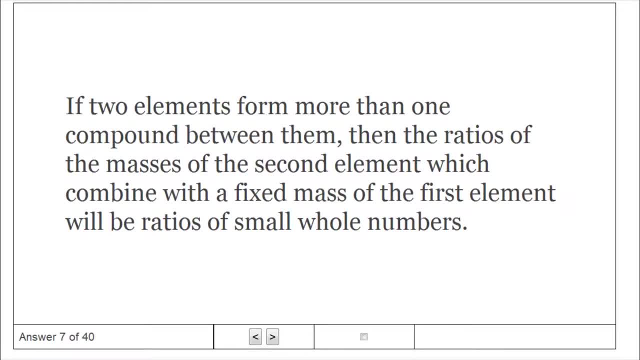 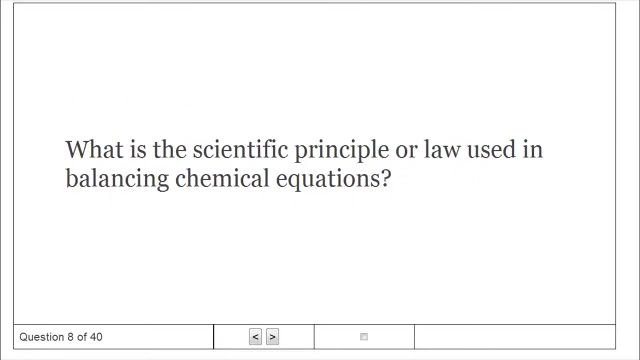 Law of Definite Proportions. The ratios of the masses of the second element which combine with the fixed mass of the first element will be ratios of small whole numbers. What is the scientific principle or law used in balancing chemical equations? Law of Conservation of Mass. 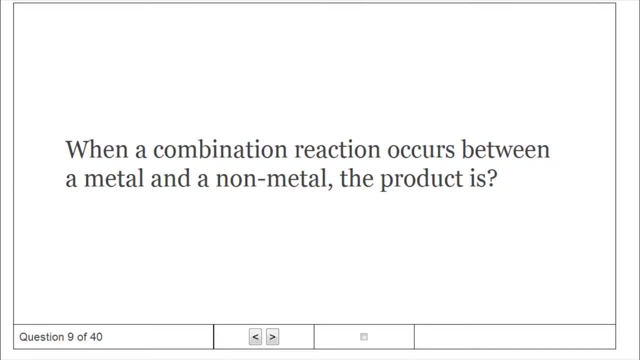 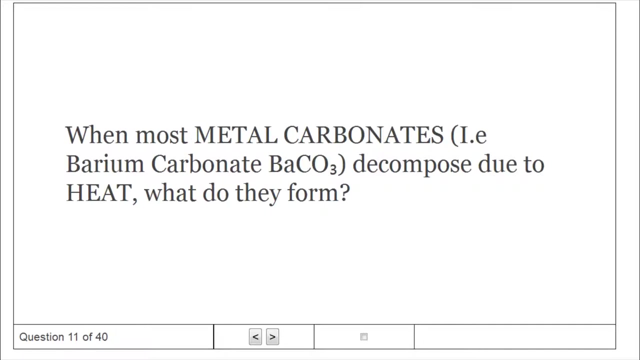 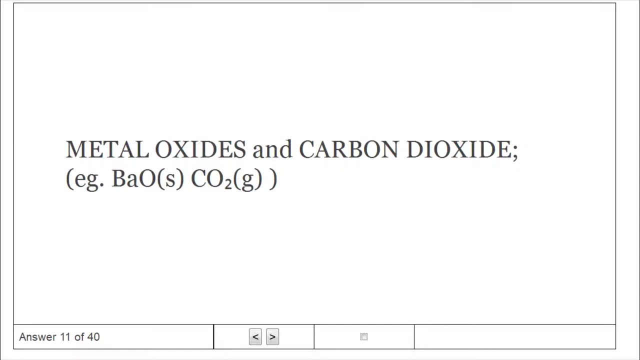 When a combination reaction occurs between a metal and a non-metal, the product is an ionic solid. Combination reactions generally form: how many products? Only one product. When most metal carbonates decompose due to heat, what do they form? Metal oxides and carbon dioxide. 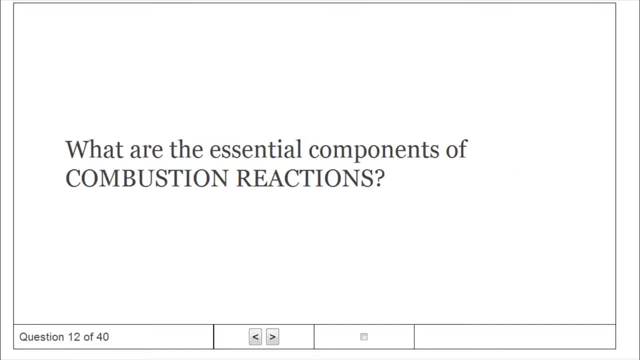 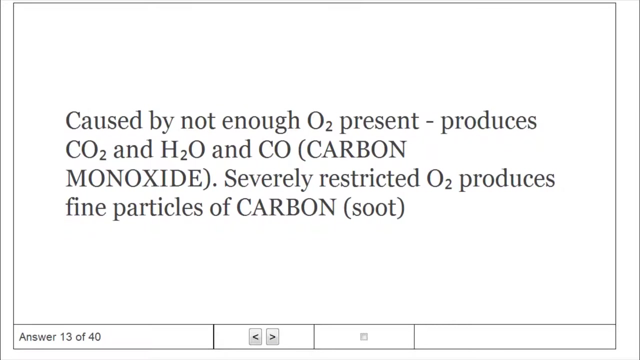 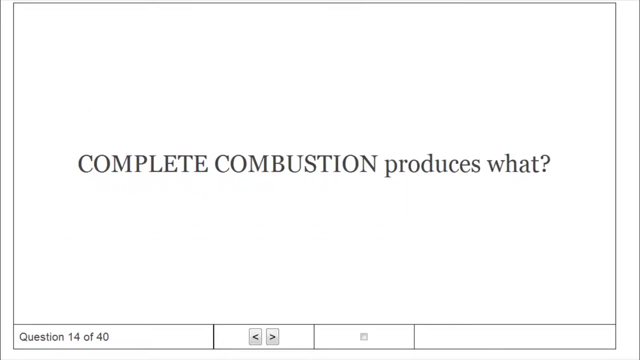 What are the essential components of combustion reactions? Rapid reactions that produce a flame. What is incomplete combustion caused by? and what does it produce? Caused by not enough O? present produces CO and HO, and CO Produces fine particles of carbon. Complete combustion produces what 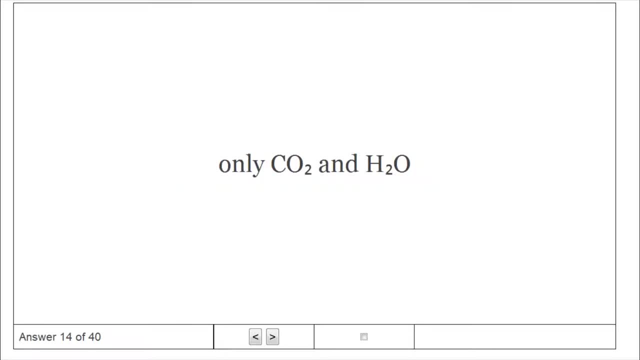 Only CO and HO. What is complete combustion caused by and what does it produce? Carbon7.. What impacts the state of the resulting water in a combustion reaction- Carbon8.. What is incomplete combustion caused by and what does it produce? Carbon9.. 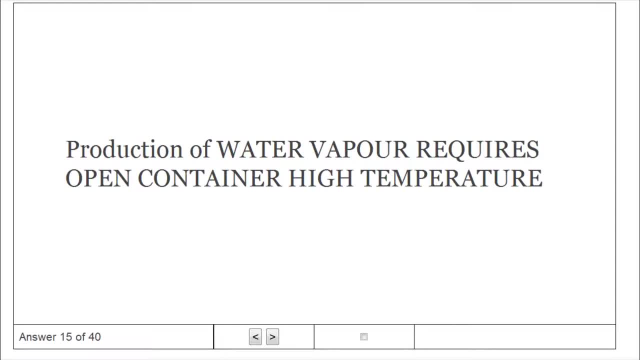 What production of water vapour requires open container, high temperature- Carbon10.. What substance in our body produces CO and HO and an oxidation reaction- Carbon11.. What means happens if the breakdown of vibration occurs in a certain разur motif? What substance in our body produces CO and HO in an oxidation reaction? 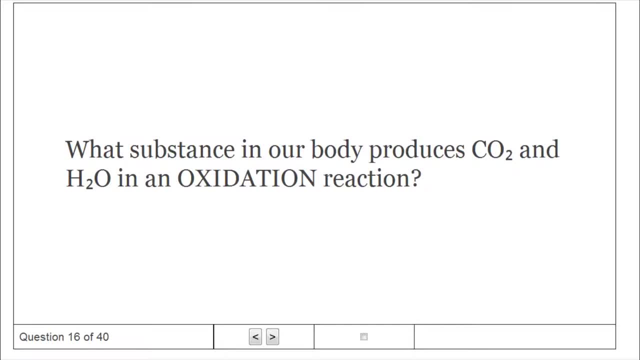 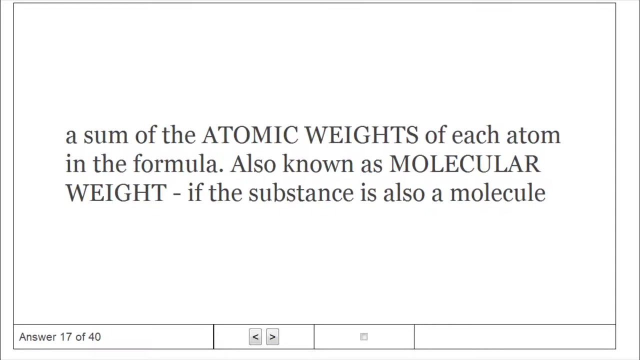 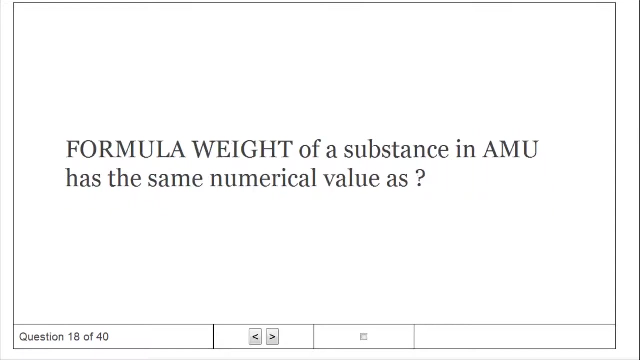 reflection, oxidation, reaction. glucose formula. weight of a substance: a sum of the atomic weights of each atom in the formula also known as molecular weight. if the substance is also a molecule, the formula weight of a substance in amu has the same numerical value as the molar mass expressed in grams. 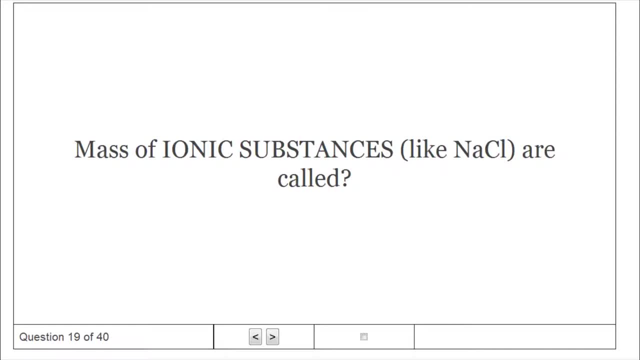 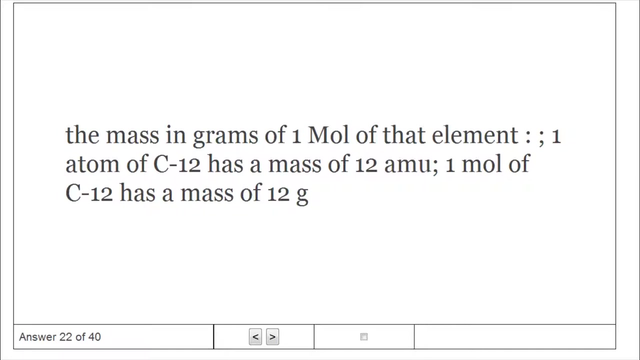 mass of ionic substances are called formula units. avogadro's number 60221421, 6 mal equals amount of atoms as there are in exactly 12 grams of pure carbon-12. the mass in amu of a single element is equivalent to The mass in grams of 1 mol of that element. 1 atom of C12 has a mass of 12 amu. 1 mol of C12 has a mass of 12 grams. 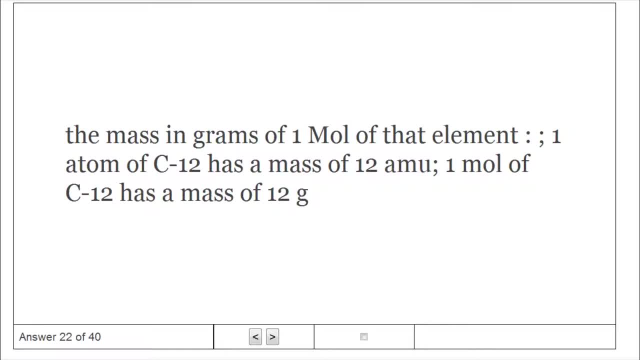 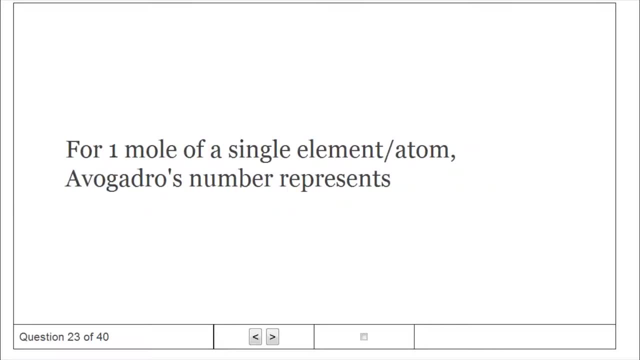 For 1 mol of a single element, atom, Avogadro's number represents number of ams. For 1 mol of a compound or molecule, Avogadro's number represents number of atoms. Number of molecules: Molar mass: Mass in grams of 1 mol of a substance. 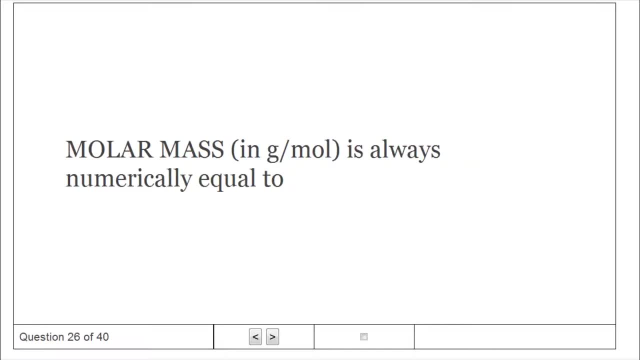 Molar mass is always numerically equal to the formula. weight. Rules for mass calculations: Grams use molar mass. Moles use Avogadro's number. formula units: How many molecules in y grams of x substance Equals asterisk: 6.022x10 squared cubed. 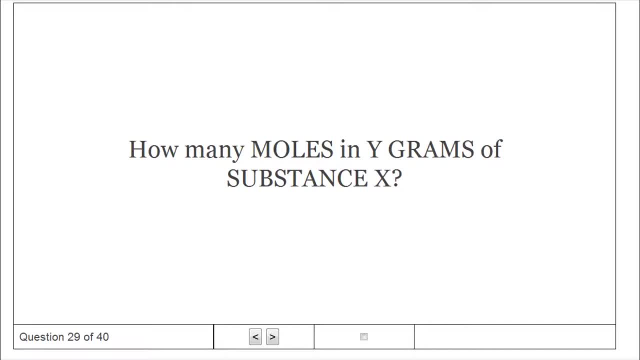 How many moles in y grams of substance x Equals How many molecules in x grams of y substance Moles y equals molecules equals 6.022x10 squared cubed. What is the mnemonic for converting percentage composition to empirical formula? 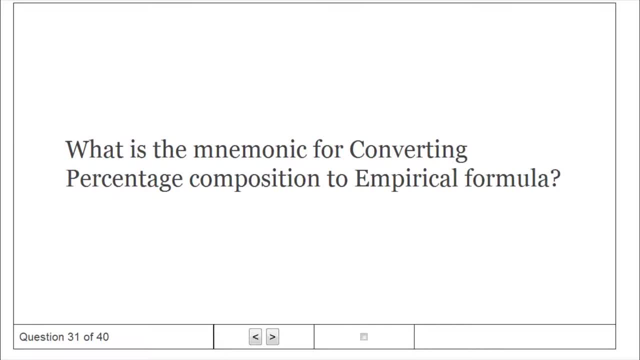 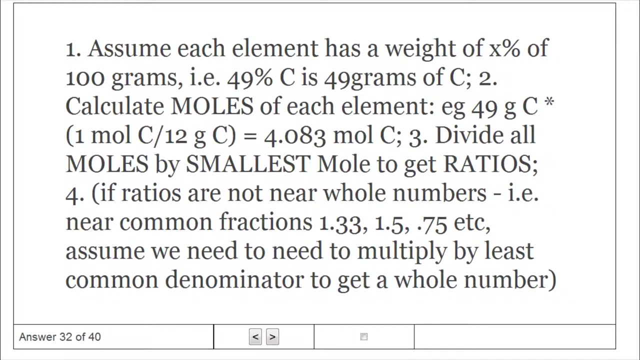 Percentage to mass, Mass to mole. Divide by small, Multiply till whole. What are the steps to covert percentage composition to empirical formula? 1. Assume each element has a weight of x percent of 100 grams, ie 49%. c is 49 grams of c. 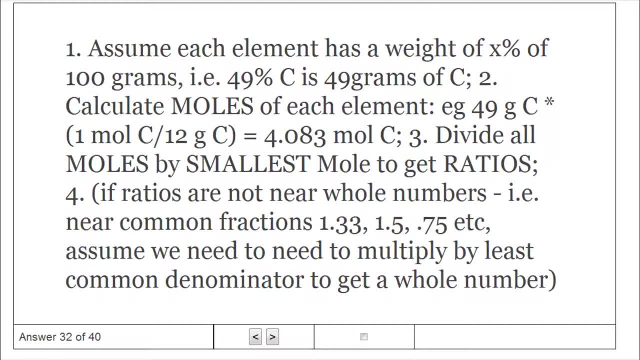 2. Calculate moles of each element. eg 49 grams c asterisk equals 4.083 moles c. 3. Divide all moles by smallest mole to get Ratios 4.. 2. Assume all moles by smallest mole to get. 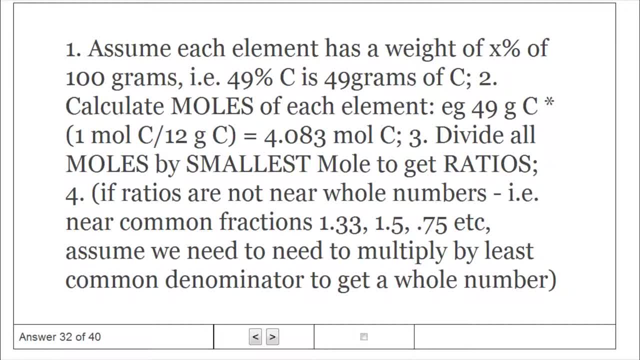 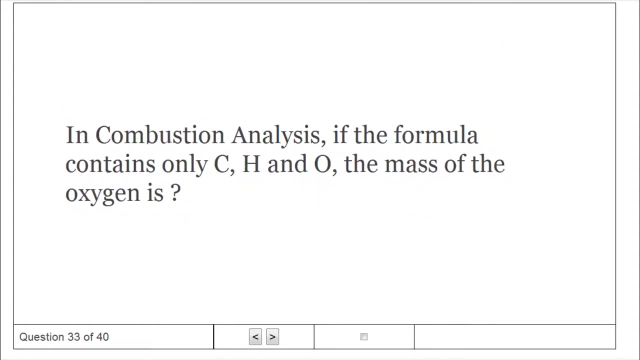 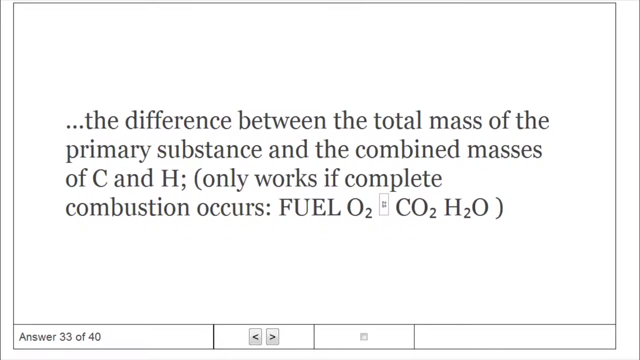 Ratios 4.. 3. Assume all moles by smallest mole to get In combustion analysis if the formula contains only c, h and o. the mass of the oxygen is The difference between the total mass of the primary substance and the combined masses of c and h. 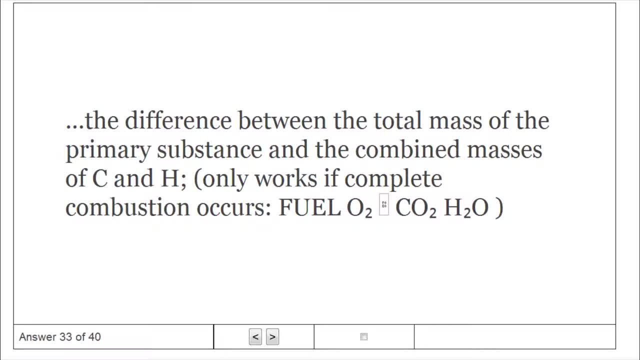 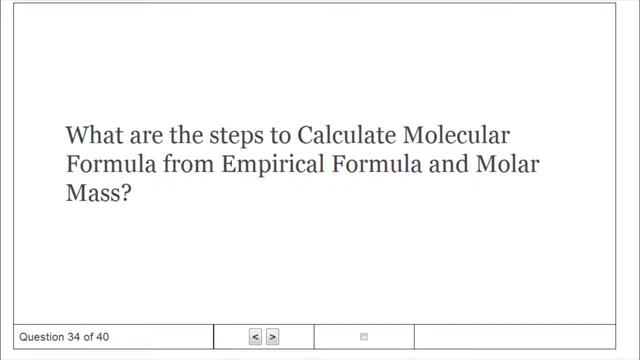 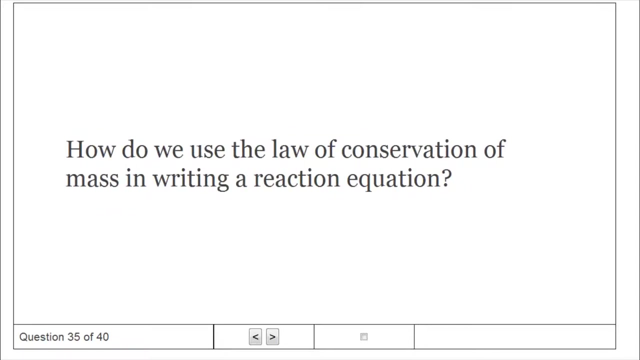 What are the steps to calculate molecular formula from empirical formula and molar mass? 1. Equals ratio. 2. Multiply empirical formula by ratio. How do we use the law of conservation of mass? in writing. a reaction equation: The total mass of the reactants must equal the total mass of the products. 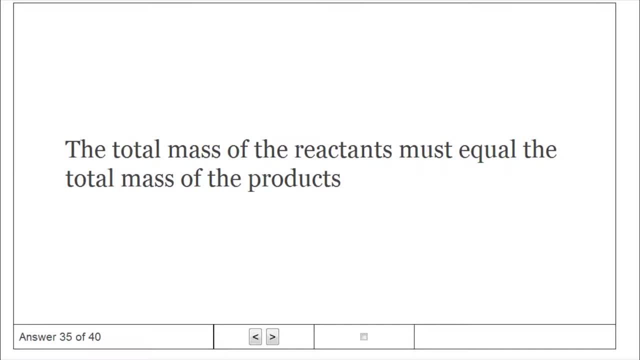 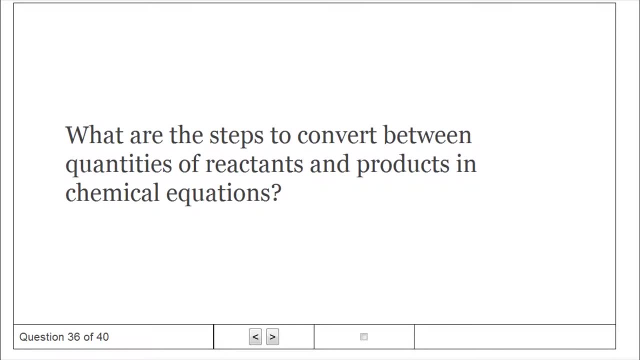 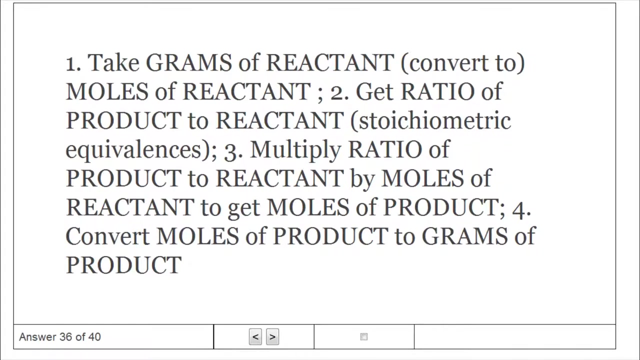 What are the steps to convert between quantities of reactants and products in chemical equations? 1. Take grams of R-E-A-C-T-A-N-T, moles of R-E-A-C-T-A-N-T. 2. Get ratio of product to R-E-A-C-T-A-N-T.